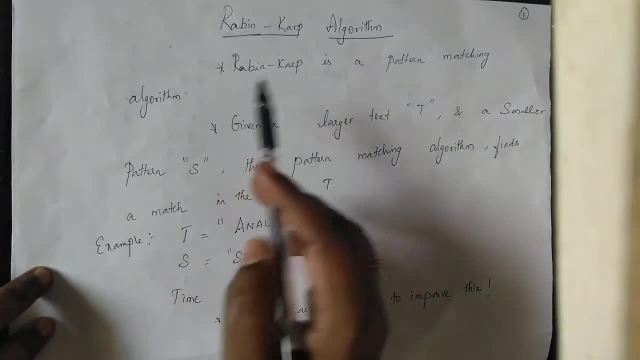 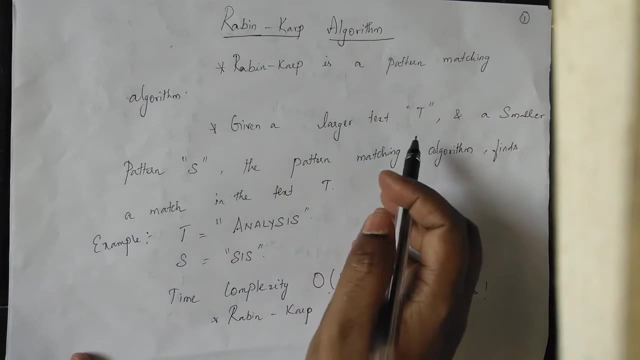 Hello all, today we are going to see about Rabin-Kopp algorithm. Rabin-Kopp is a pattern matching algorithm, So first we need to understand what is pattern matching. So, when we are given a larger text in terms of its length- t- and a smaller pattern, s, so the pattern matching algorithm. 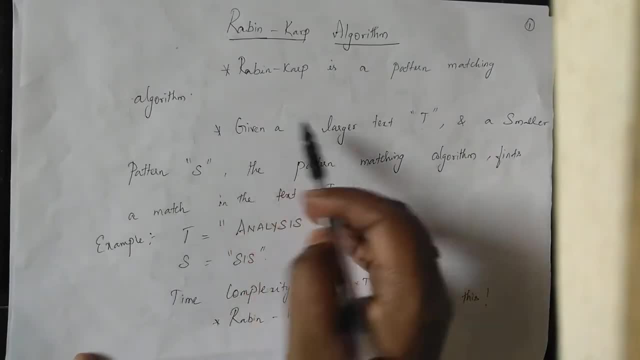 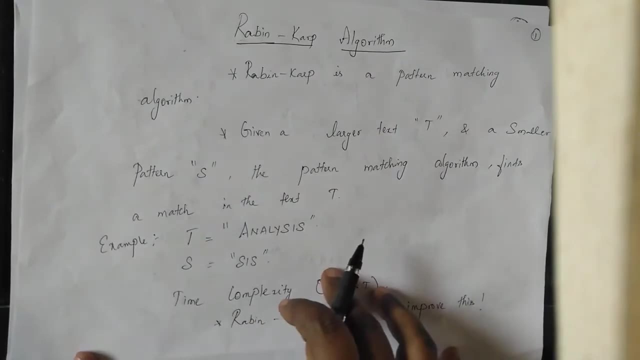 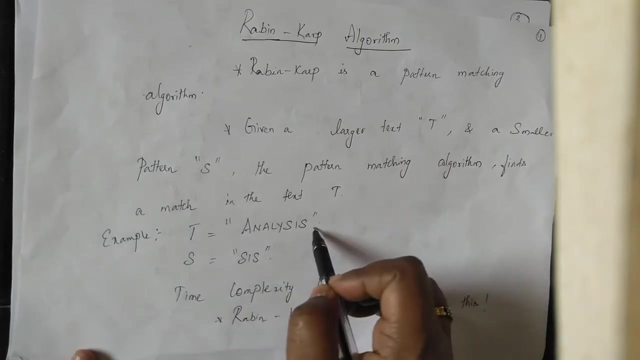 finds a match in the text t. So with this it tries to find how many number of times this pattern has occurred in this t text t. So that is what a pattern matching means. So we will see through an example. So let us say the text t is analysis. So in real time application this would be a 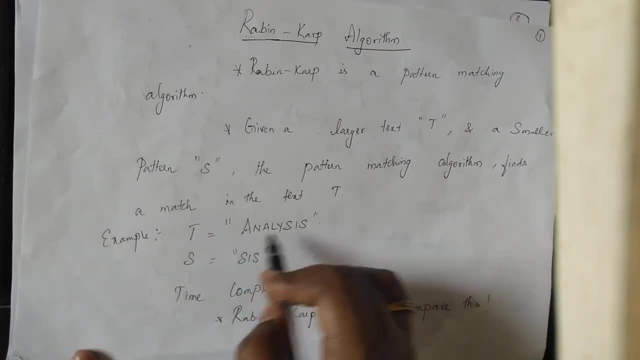 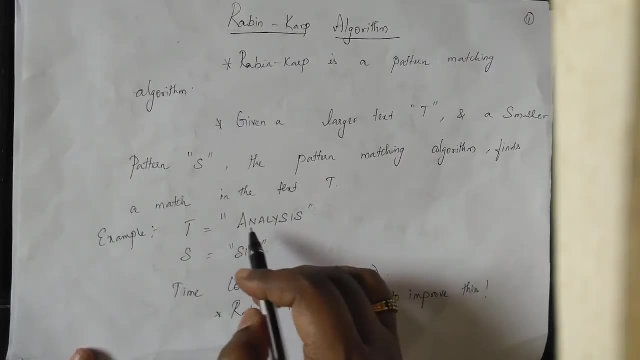 larger, this will be of larger length. So for simplicity I have given a single word: So and the pattern s is. so the pattern matching algorithm tries to find the match between this pattern and this text. So how many number of times this pattern has occurred in this t? So this is a? 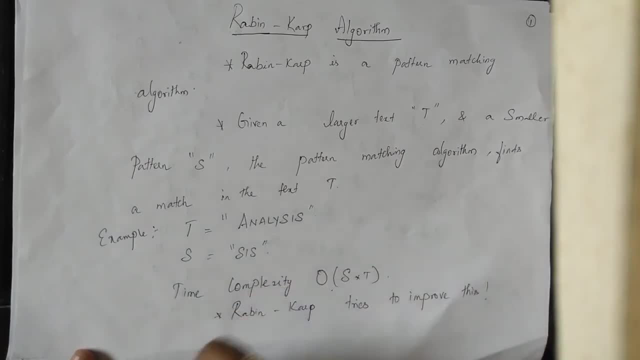 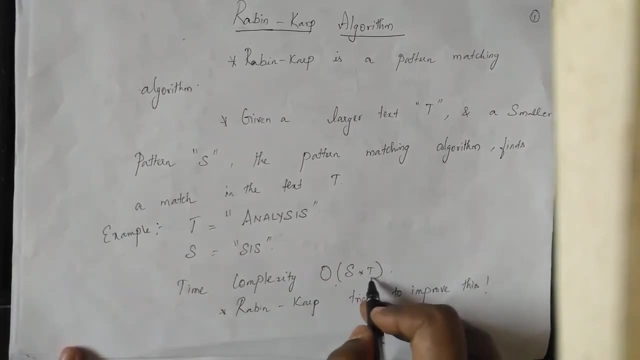 pattern matching algorithm. So the worst time complexity thrown by such pattern matching algorithm is big O of s into t, where s is the length of the pattern and t is the length of the text. Rabin-Kopp algorithm is one such kind of pattern matching algorithm which tries to improve. 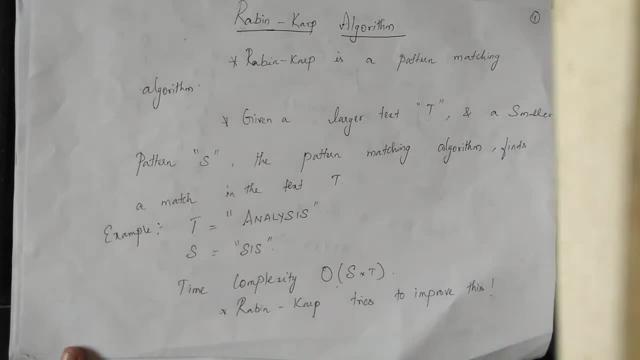 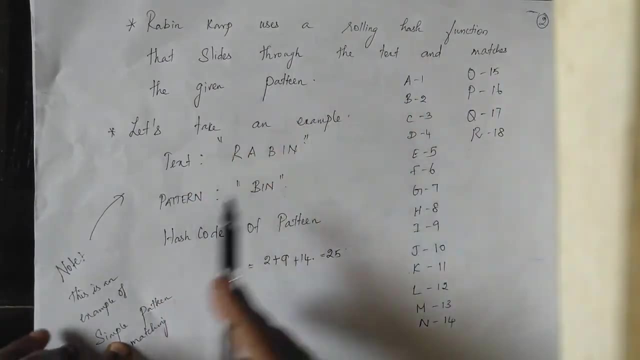 this time complexity. So that is what we are going to see about today. So all these pattern matching algorithm, you should know that they are not just a pattern matching algorithm, So this is a rolling hash function So that we will understand shortly. So we will take an example and 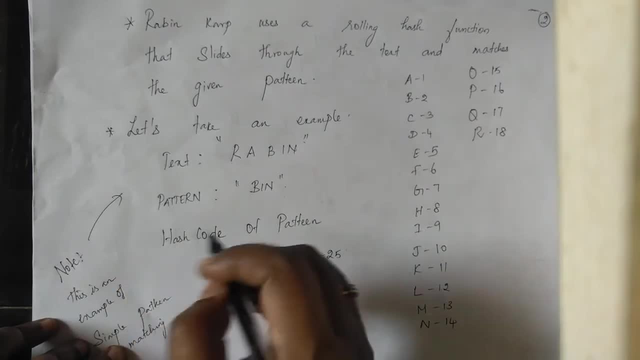 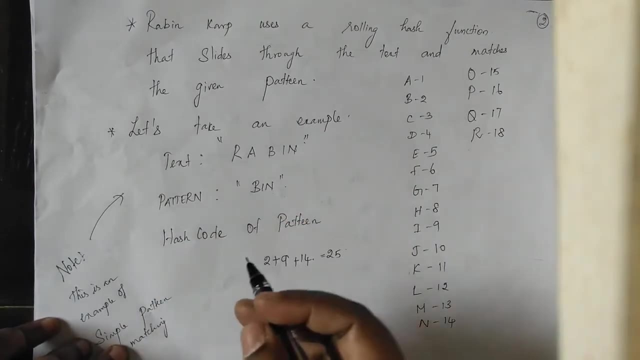 see actually how this pattern matching algorithm works. Let us say the text is Rabin this time and the pattern is Bin, that is, Bin this time. So how they find a match is that. so they compute the hash code of this Bin and they slide through the characters in the text, from the first character. 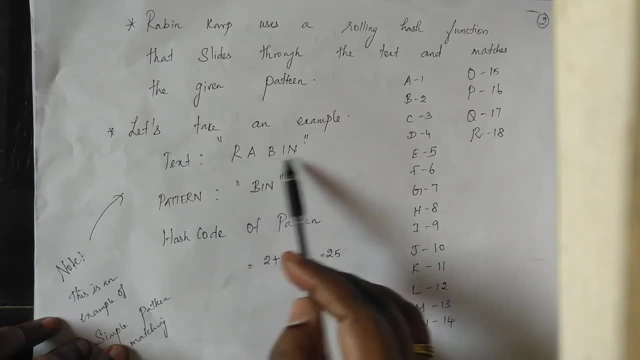 whether this hash code is present in this text or not. They compute three hash code values for three, three characters and they slide through this text. Why? Because the length of the pattern is three. So that is why we take three, three characters. First. we will try to find the 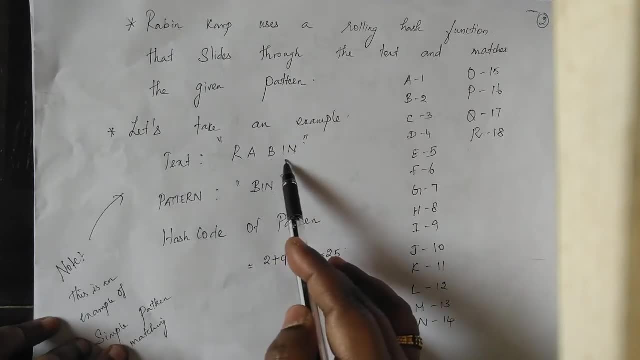 hash code of Rab, and then we will try to find the hash code of Abi, and then we try to find the hash code of Bin, and then we try to find whether the pattern is present or not. So, as a first step of finding the pattern, we need to find the hash code of the pattern. So that is what we need to do. 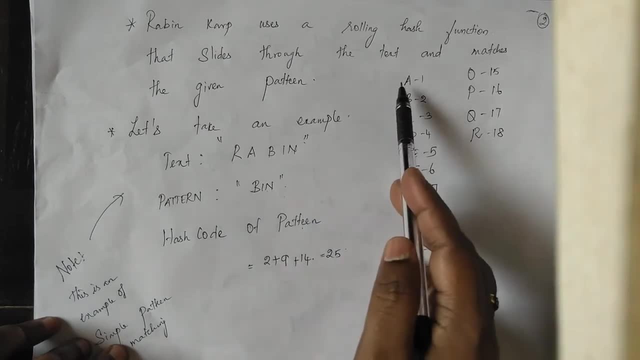 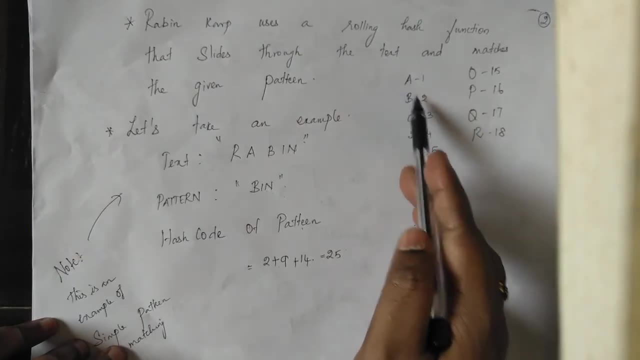 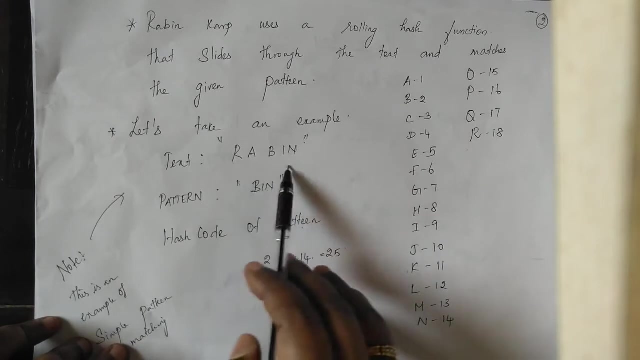 first To find the hash code. so normally hash code uses the ASCII value of these alphabets. For simplicity I have taken a simple number coding: A is mapped with 1 and B is mapped with 2 and so on. So we have shown. I have shown only till R. why? Because the example demands till R only. So. 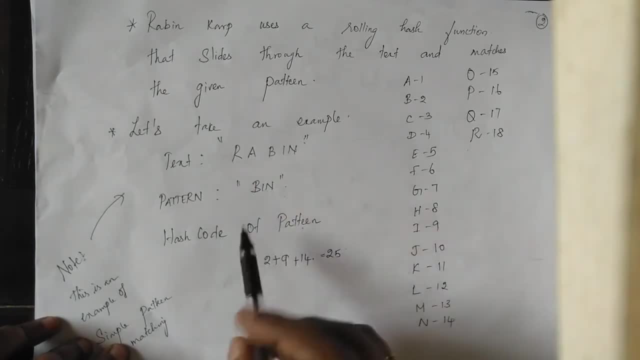 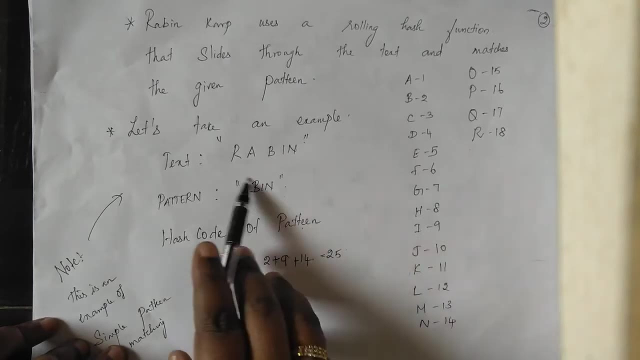 otherwise we could have taken the entire alphabets. Okay, so now the B's value is 2, so B is coded with 2 and I is coded with 9 and N is coded with 14.. So when we add them together, 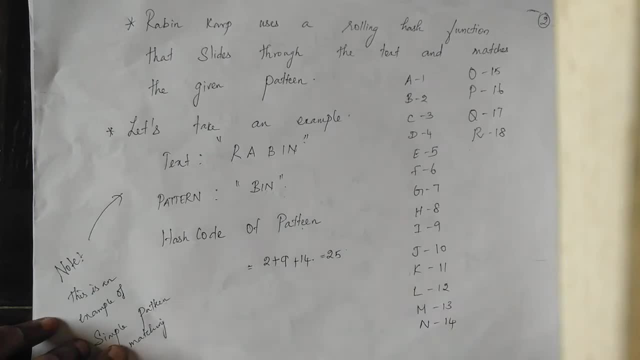 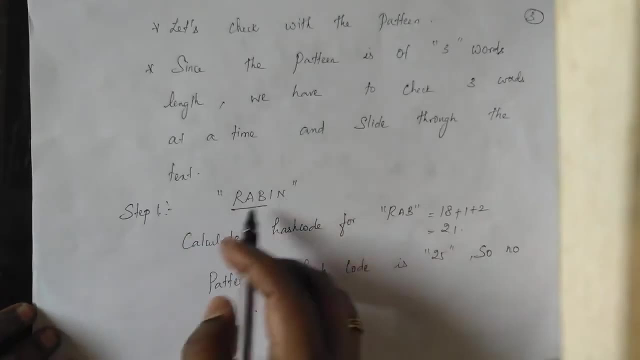 we get the hash code to be 25.. So now we have to slide through the text and we have to see whether the text is present or not. As a step 1, we will see that in step First we have to check. 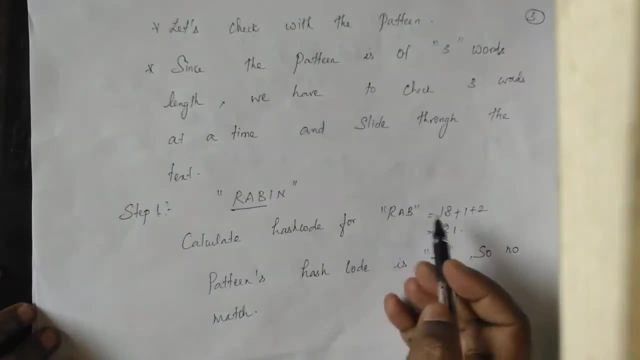 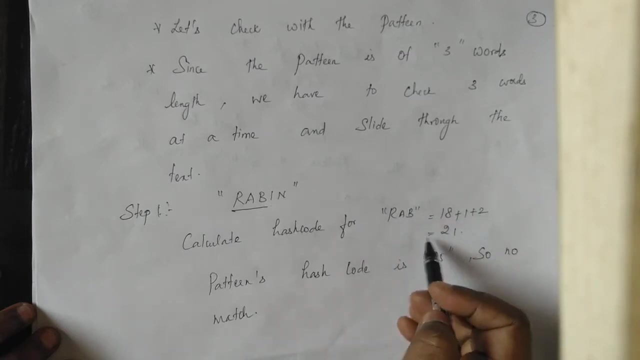 Rab. We have to compute the hash code of Rab. R's value is 18 and A's value is 2 and B's value is 2.. Sorry, A's value is 1 and B's value is 2. We get when we add them together. we get 21.. So our 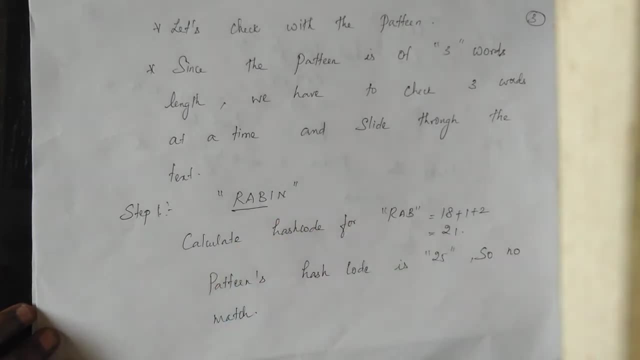 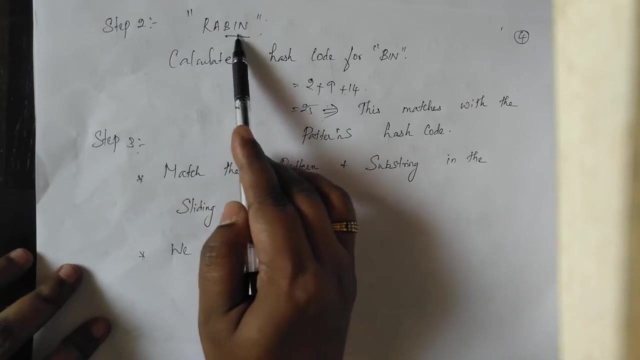 pattern's hash code was 25.. So this is not our pattern. So now we have to check for ABI. I'm sorry, I have skipped that step here. So in the second step we actually need to have computed the hash code of ABI. I've directly come to BIN, So I've skipped that step, Sorry. So now here we. 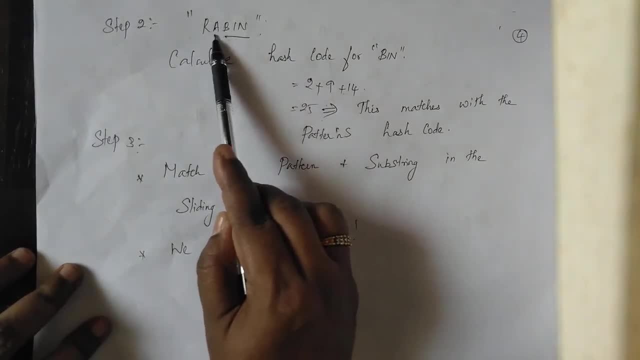 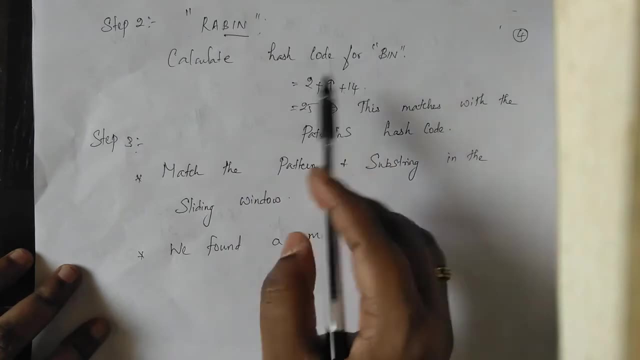 are calculating after having computed the hash code of ABI. ABI is hash code. We have to move to BIN, So that is what is shown here. So when we calculate the hash code of BIN, so B's value is 2, I's value is 9 and N's value is 14.. We add them. 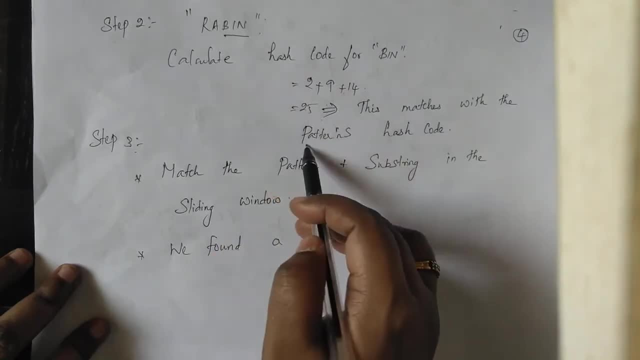 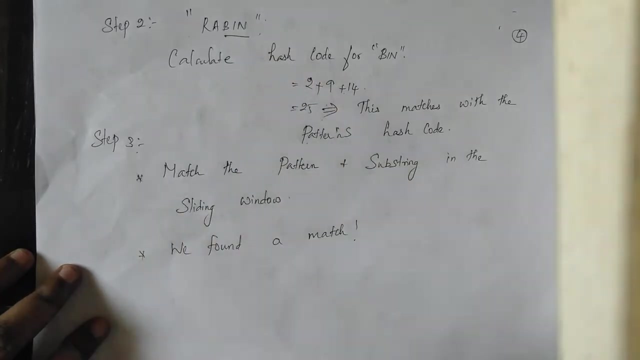 we get 25.. Actually, our pattern's hash code was 25.. So we cannot stop here. We need to actually match them. So whether this is a hash code, match, but we need to find the actual string match. So of course there is a match, because our pattern was BINs and we have found a match. 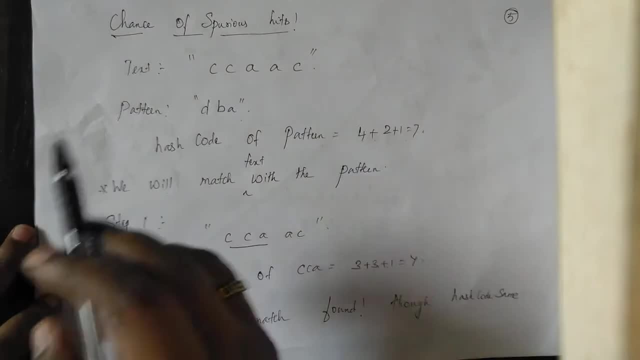 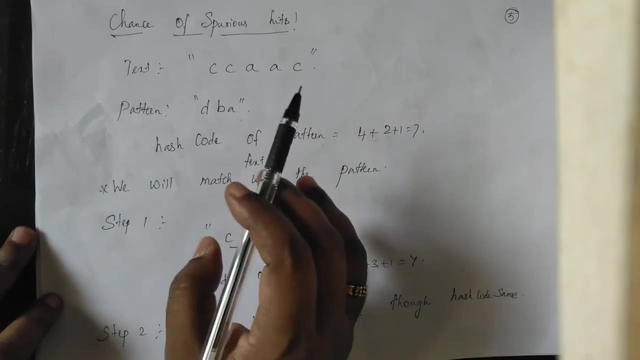 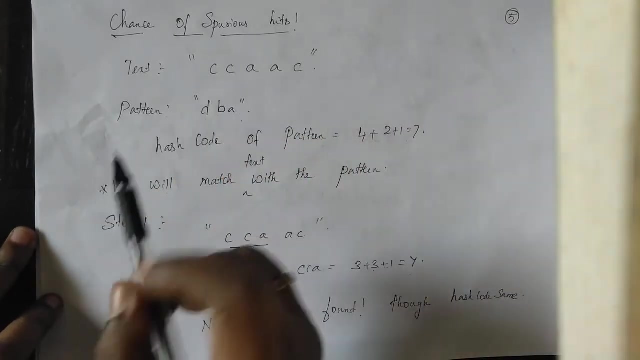 So here comes the disadvantage of such a pattern: a simple pattern matching algorithm that was not a RobinCop pattern matching, So that's a simple pattern matching algorithm that we discussed till now. So that has a disadvantage of spurious hits. We'll understand what is that. 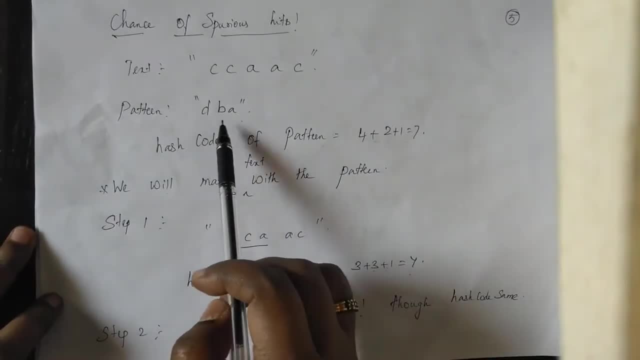 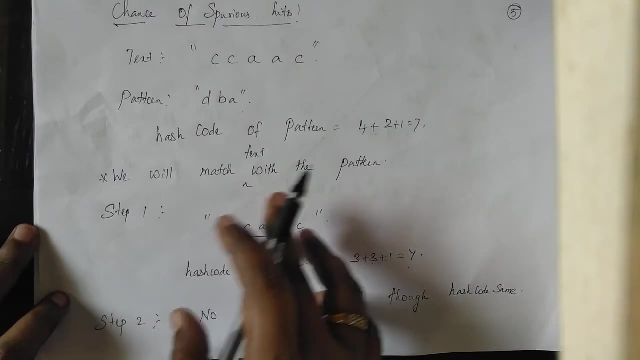 Let's take this text- CCAAC- and let's take this pattern- DBA. So we'll find whether this pattern has present in this text or not, using the hash code. So let's take this text- CCAAC- and let's take the hash code we discussed earlier. So when we find the first, we need to find the hash code of. 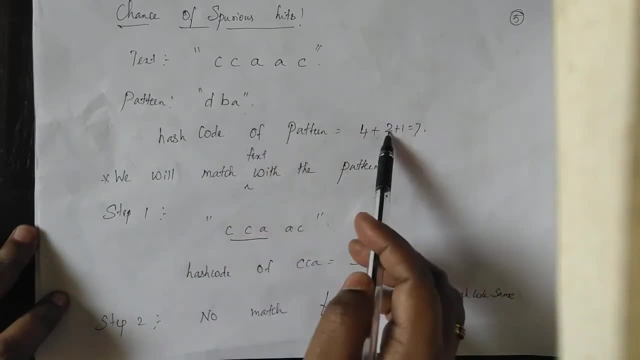 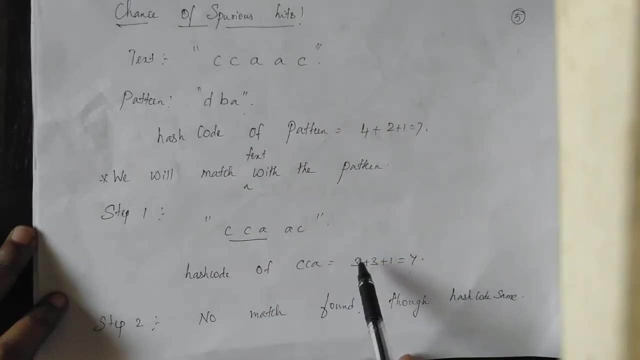 the pattern. So D's value is 4, B's value is 2 and A's value is 1, we get 7.. So in step 1, when we look at the first three texts, C's value is 3 and C again 3 and A's value is 1, we add them up and 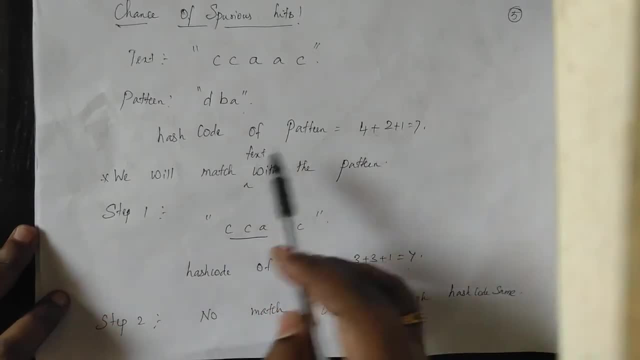 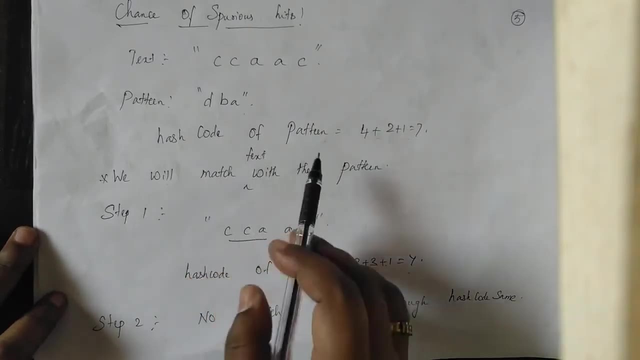 we get the 7. So that is a hash code match. But when we try to find the string match, they don't match. This is what we call it as spurious hits, When these kind of spurious hits occur frequently. so then that is going to. 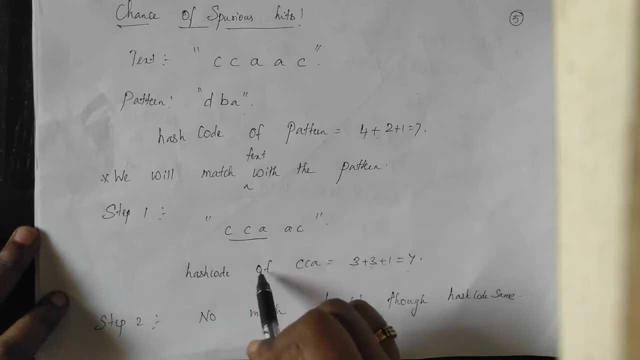 worsen the time complexity. This is happening why? Because the hash code, what we computed- is weaker, So we need to strengthen that and that's what Rabin Kopp algorithm proposes- That comes up with a stronger hash code. So we'll see that how that works. 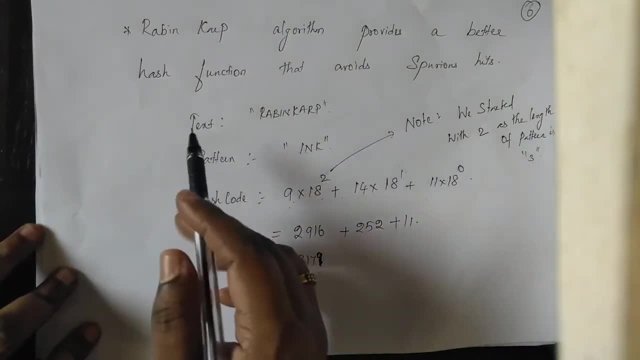 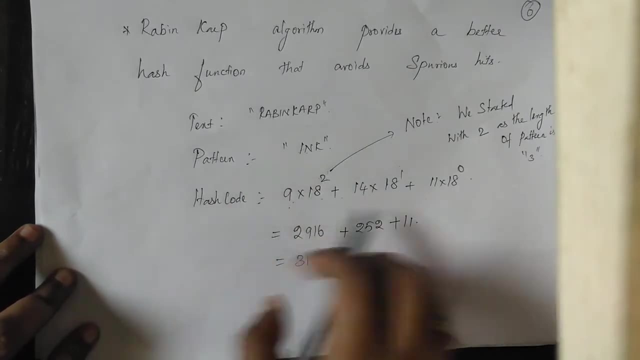 Yeah, so this is how Rabin Kopp is going to work on pattern matching. So let's take this time, Rabin Kopp as the text and the pattern as INK ink. So this is how the hash code is calculated. So I is, I's value is 9.. So we have multiplied that with 18.. So why? Because we had 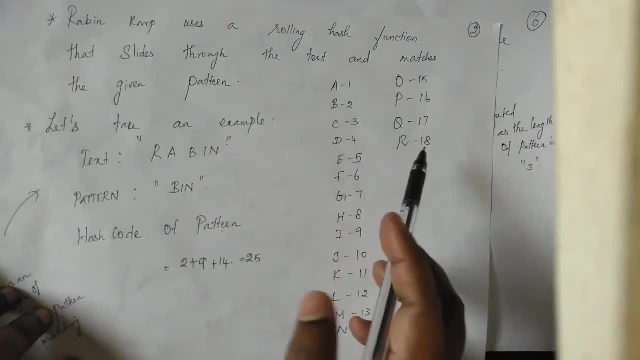 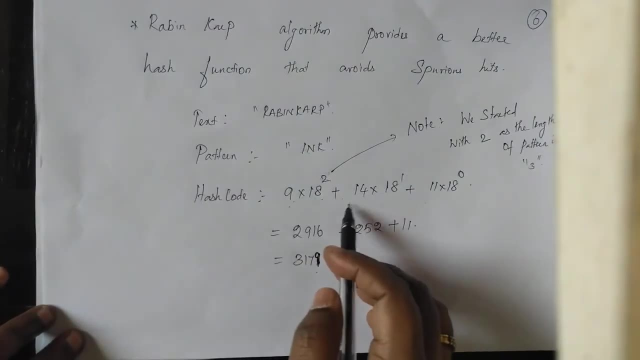 taken 18 alphabets, So that's why we had taken 18.. So we have taken the whole alphabet. we could have taken 26.. So 18 to the power of 2 plus 14, the 14's value is n and multiplied by 18 to the. 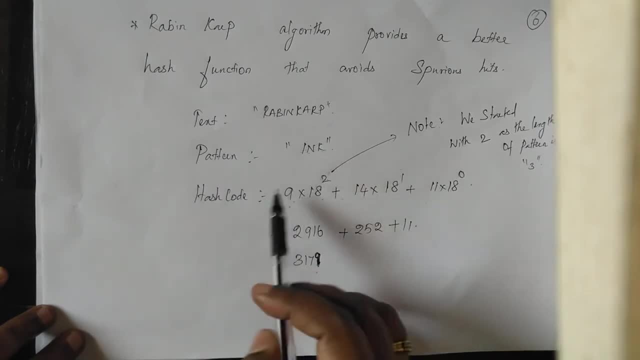 power of 1 plus a case value is 11 into 18 to the power of 0.. Okay, So this 2, we should understand why we have given we started with 2, 1, 0. So because the length of the pattern is 3, so that's. 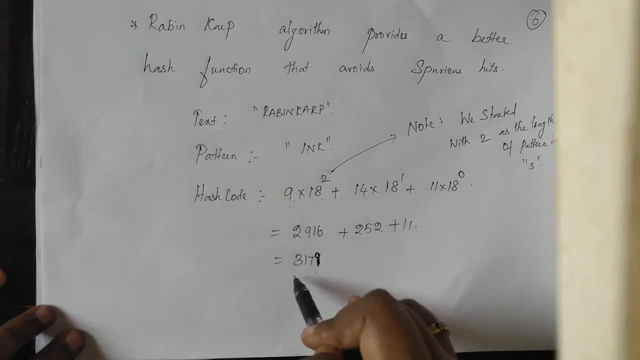 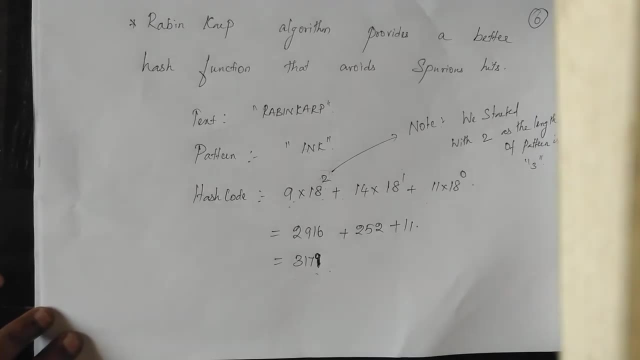 why we started with 2.. So we compute this and we get the value as 3, 1, 7, and sorry for the confusion here. That is, the value is 3, 1, 7, 9.. Now we have to slide through the text as we did. 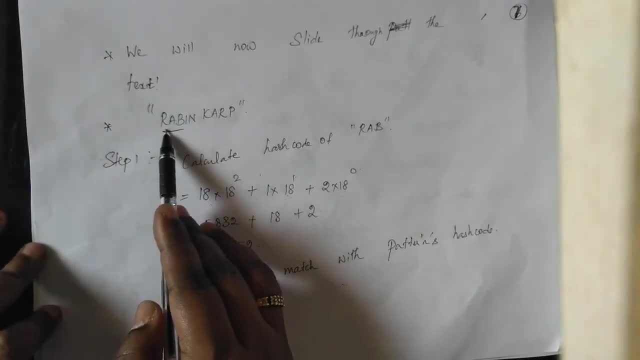 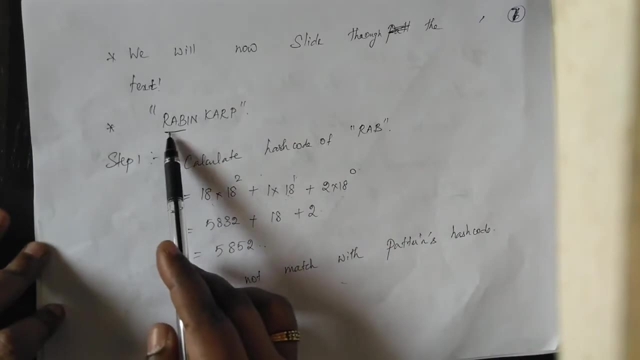 earlier and we have to find the hash code. So first we have to find the hash code of RAB. So first 3 characters. remember the length of the pattern is 3.. So that's why we are interested in finding the first 3 characters. So first we need 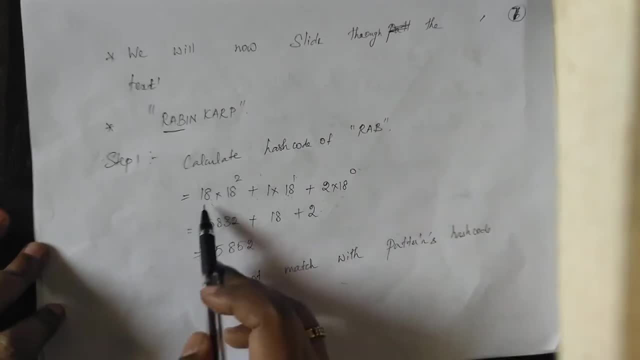 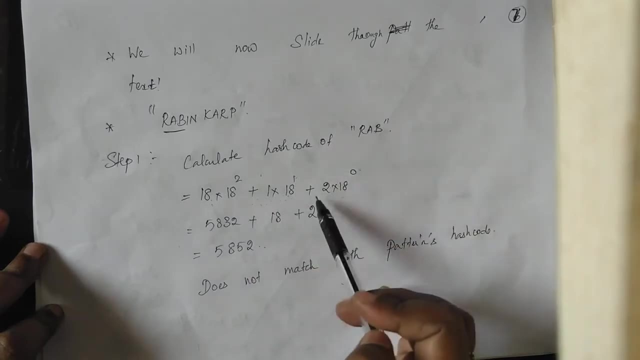 to now. we need to calculate the hash code of RAB. So R's value is 18 multiplied by 18 to the power of 2 plus A's value is 1 into 18 to the power of 1, plus 2 into 18 to the power of 0. So when we do, 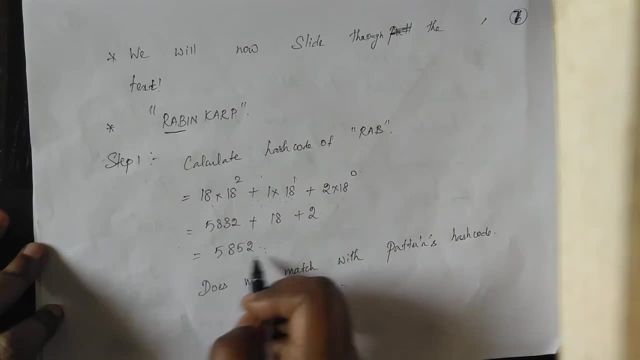 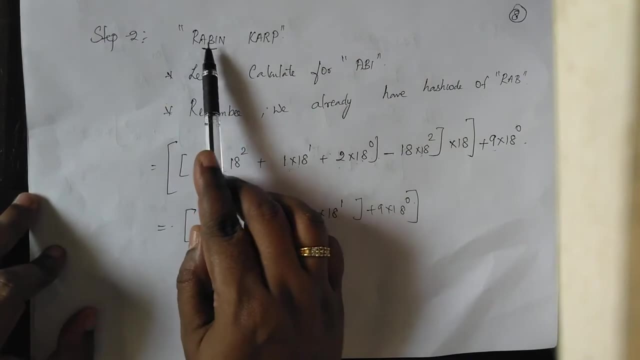 this we get value of 5, 8, 5, 2.. Obviously, this is not the value of our patterns hash code. Yeah, in the step 2, we have to slide through the text and we have to find the value of. 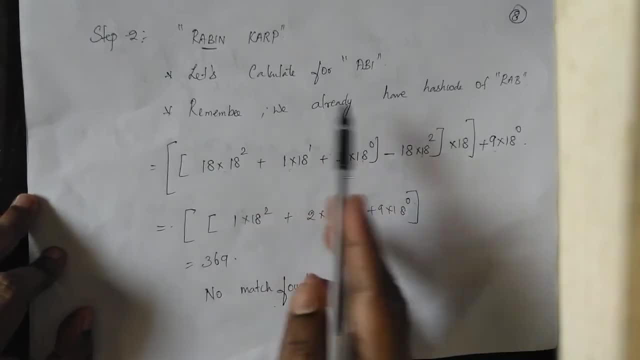 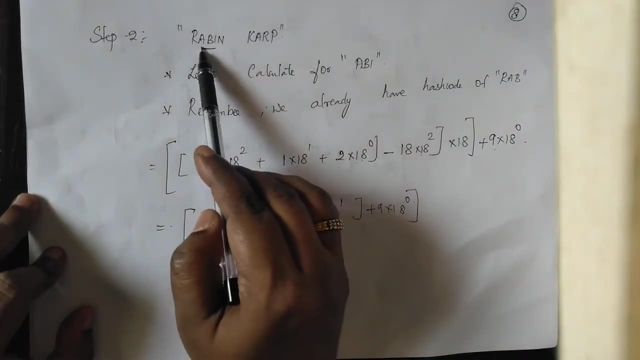 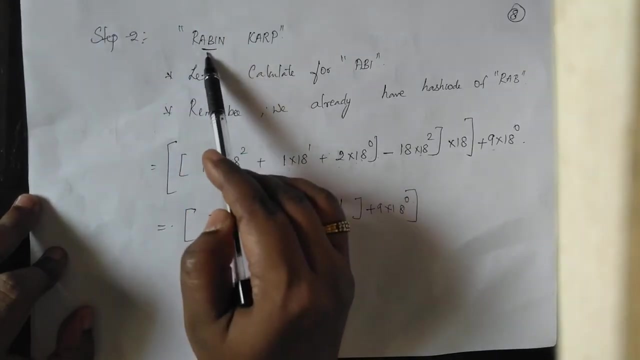 hash code of ABI. So remember, while calculating the hash code of ABI, we already have the hash code of RAB. So this is our hash code of RAB. So now we have to. when we slide through to from RAB to ABI, all we need to do is that we have to remove R and we have to include I. So this is. 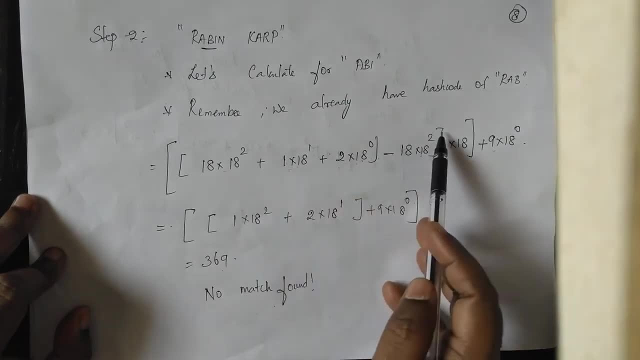 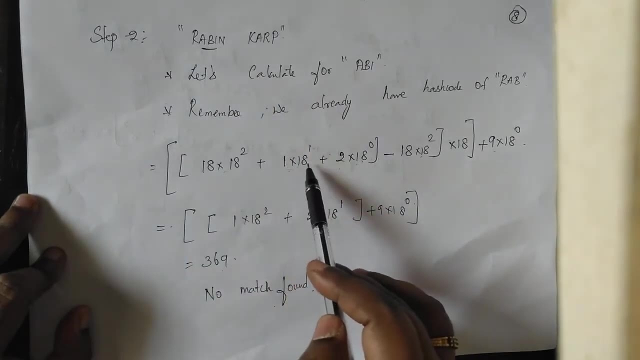 subtracting R's value. and when we subtract R's value this goes off. But to calculate the hash code of ABI, so A's value needs to be 1 into 18 to the power of 2.. So and B's value needs to be: 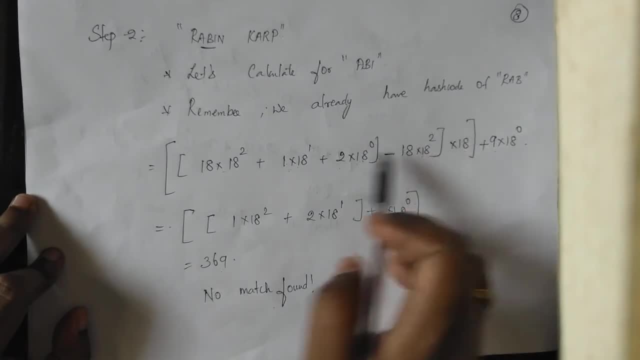 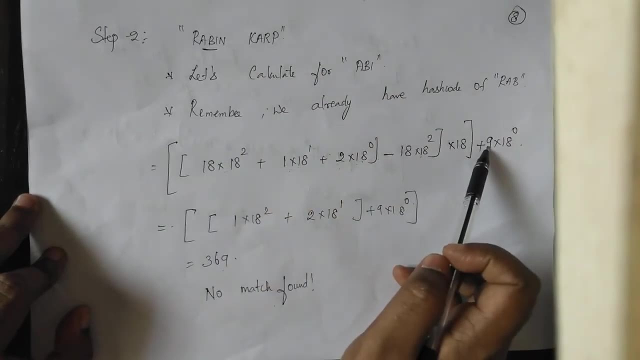 2 into 18 to the power of 1.. So we need to take 18 inside and multiply with them and we need to add I's value. So I's value is 9 into 18 to the power of 0. So that is what we get. 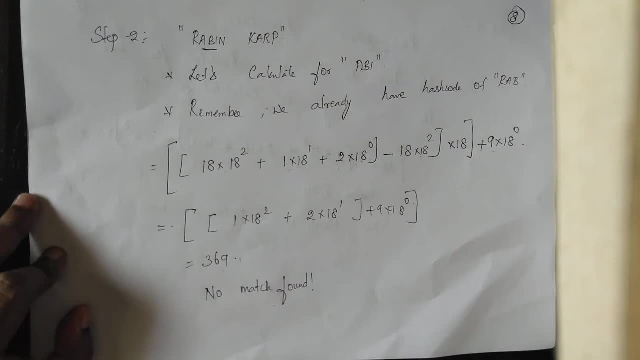 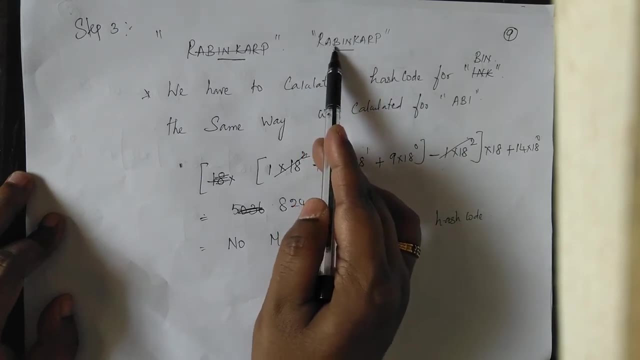 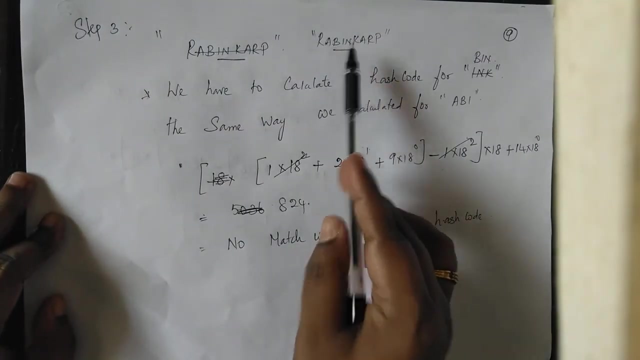 And we get 369.. So still we have not found a match. In step 3, we have to find BIN. So first we started with RAB and then we slide it to find ABI, Now BIN. So now we have ABI's hash. 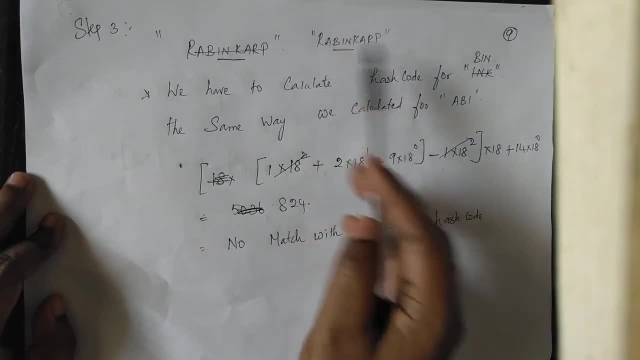 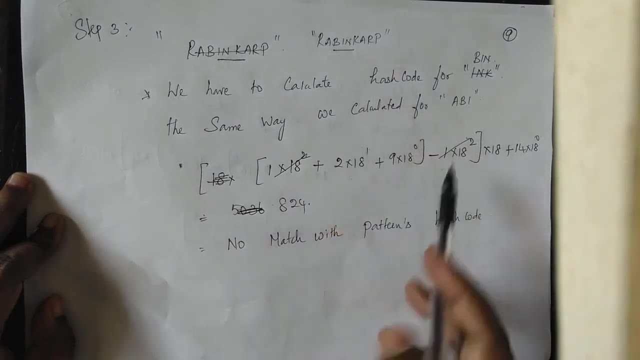 code with us. This is the hash code of ABI. We need to subtract the value of A, So this is subtracted, the value of A, and then multiply with 18.. So that is what we have done. And we have to add the value of A, So this is subtracted, the value of A, and then multiply with 18.. So that is. 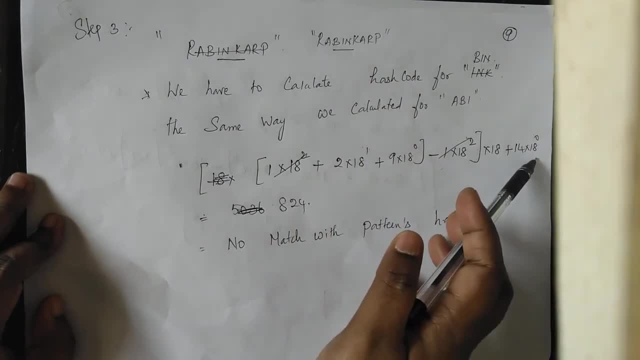 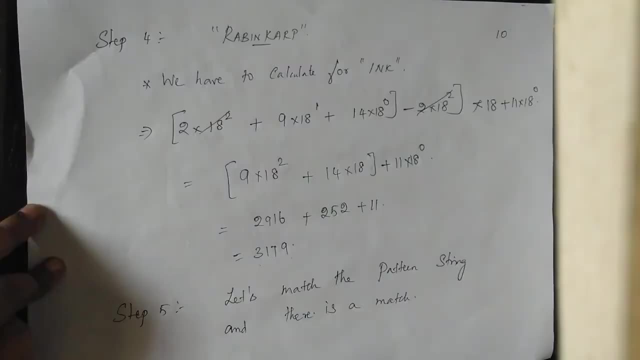 add N's value, So, which is 11 into 18 to the power of- I'm sorry, that is 14 into 18 to the power of 0. So that is 824.. Still, we have not found the match. So now, finally, we have moved to INK, So 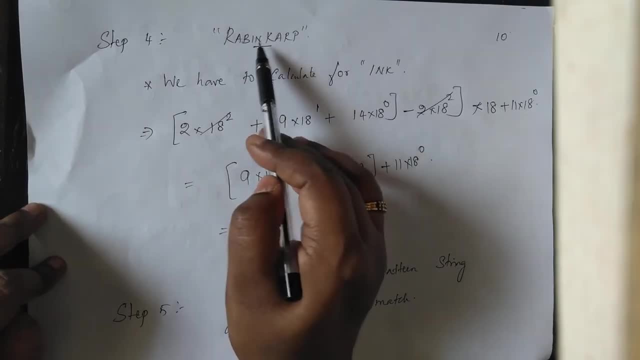 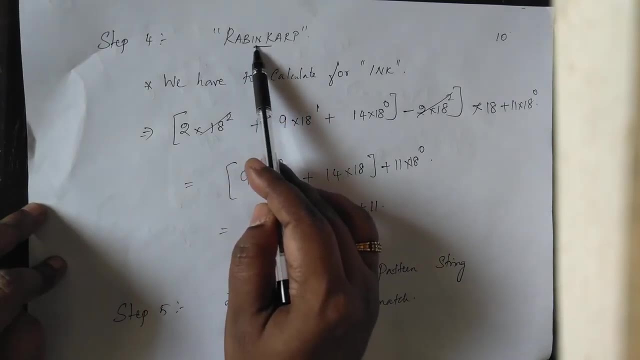 INK. that is yeah, so we need to find the. we started with RAB and then we then proceeded to ABI and then BIN. Now we are in INK. So we have to calculate the, we have to calculate the. 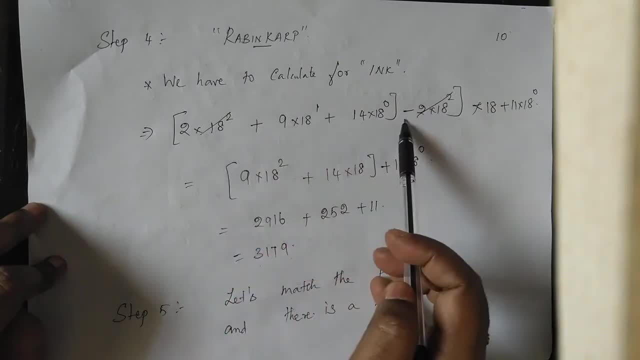 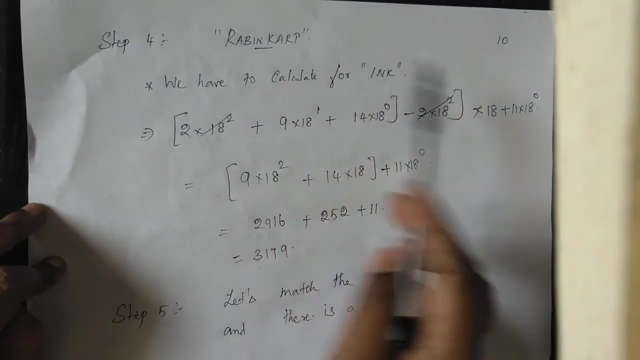 hash code of INK, So already we have the hash code of BIN. So we need to subtract the B's value from this and multiply with 18 and adds, add K's value, add K's value. So then we get 3179.. This is. 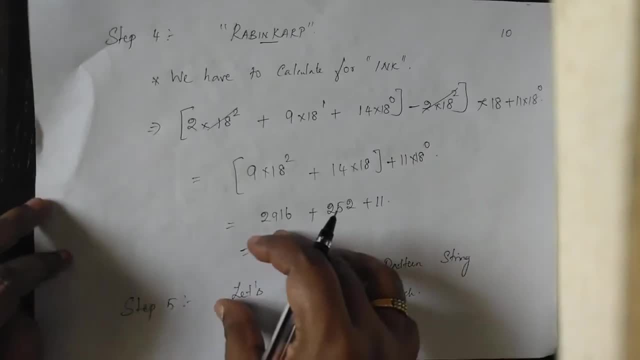 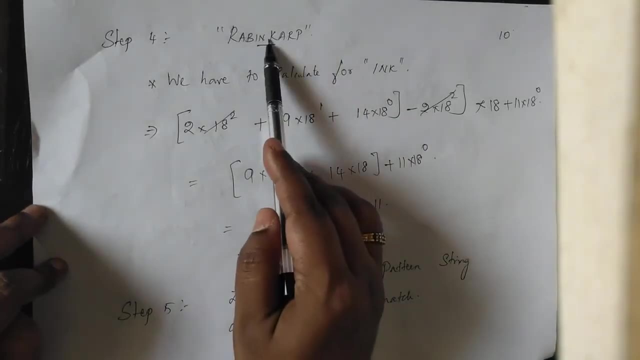 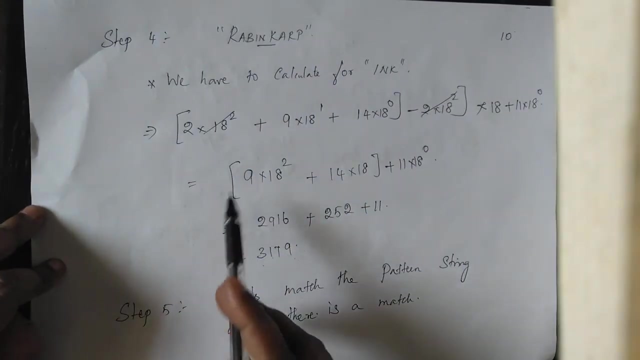 actually the hash code of our pattern. So we cannot stop here. We need to actually match the pattern with the texture. So of course our pattern was INK and we match. So we can repeat this a number of times throughout the texture. So here we are done. So 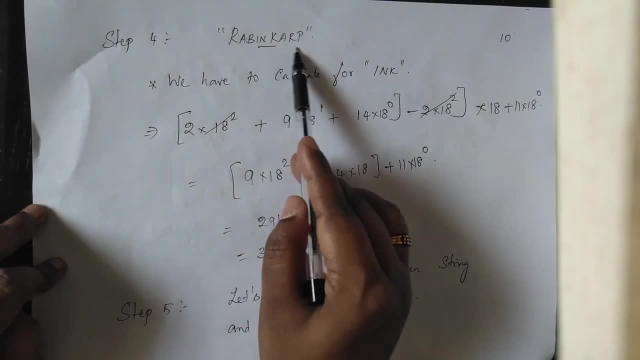 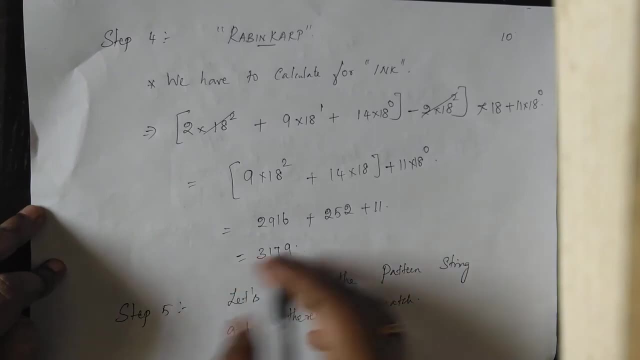 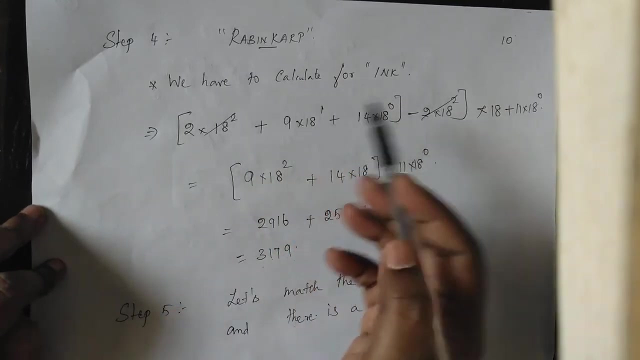 we can. we cannot stop here. We actually need to proceed for KAR and then ARP, So, but I'm stopping here for simplicity, That's understood. So in the real-time application we need to run through the entire text and we need to count how many number of times this INK has occurred.